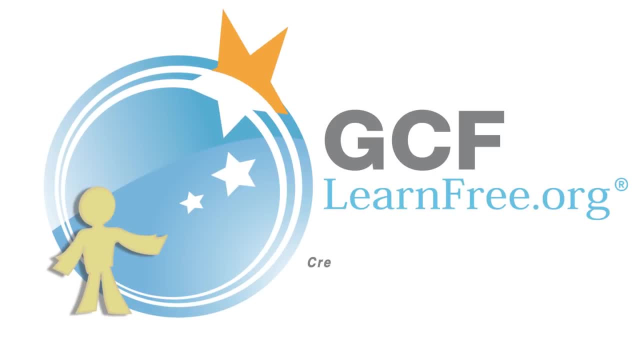 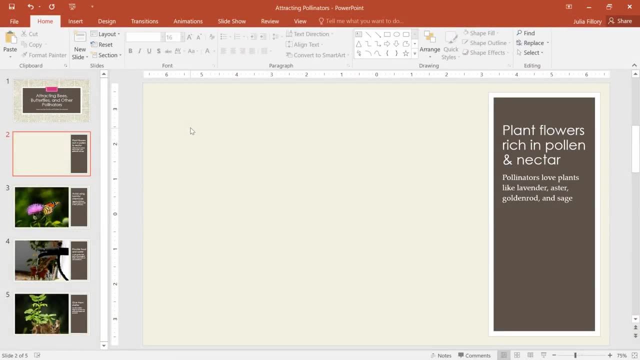 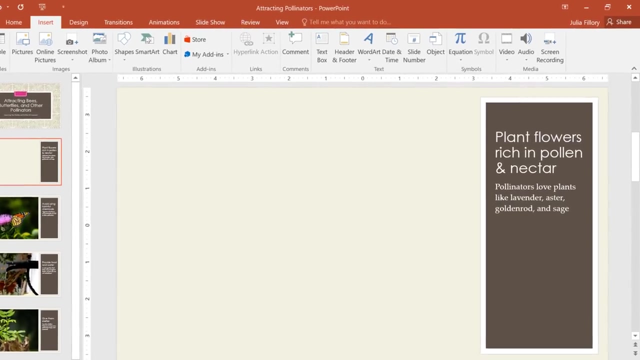 Sometimes you may have a video that you want to play during your presentation. Well, the good news is you can add the video directly to one of your slides so you can share it with the audience without having to leave PowerPoint To get started. go to the Insert tab, then look for the Video command on the far right. 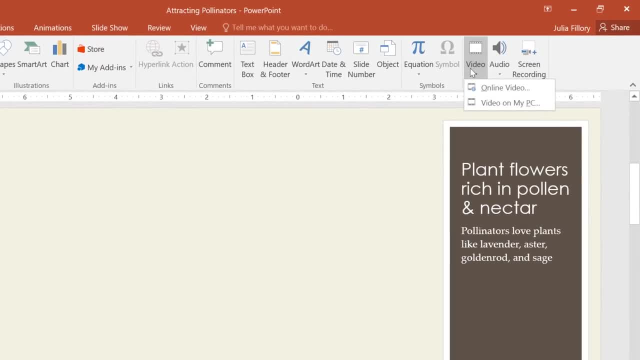 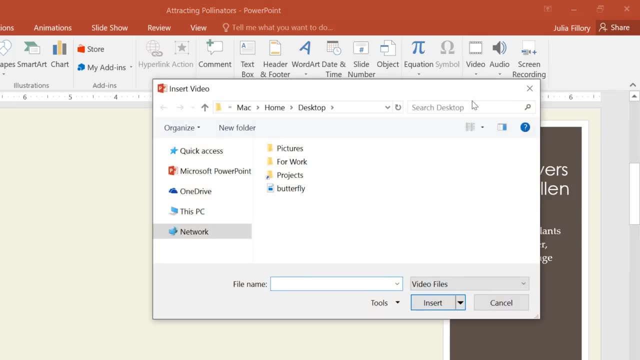 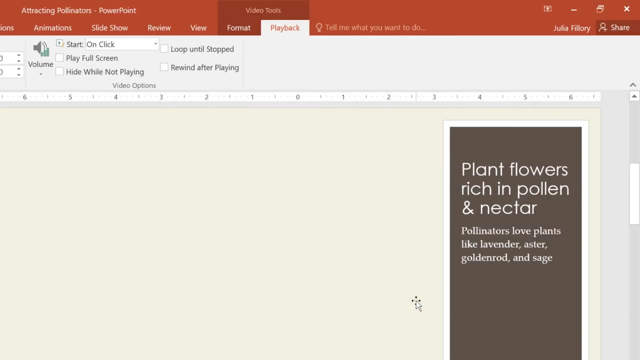 of the ribbon. From here you can insert a video from the web or one that's saved to your computer. In this example, we're going to choose the second option. Next select the file you want, then click the Insert button and the video will be added. 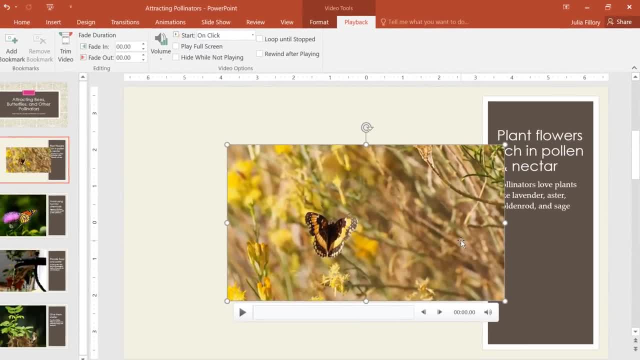 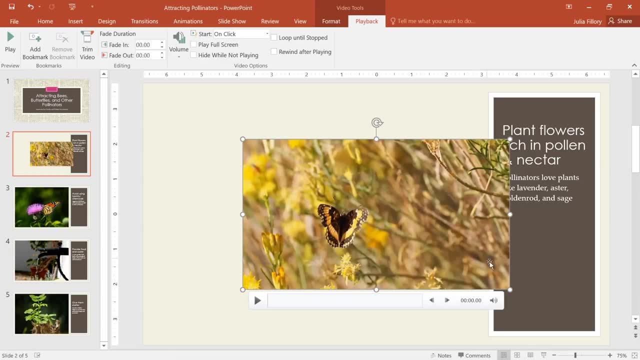 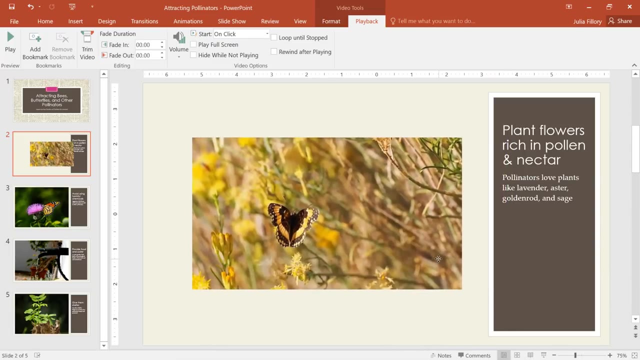 to your presentation. If the file size is very large, it might take a minute to finish uploading. Just like pictures, videos can be moved and resized any way you want. You can use the sizing handles on the sides or in the corners and then just drag and drop. 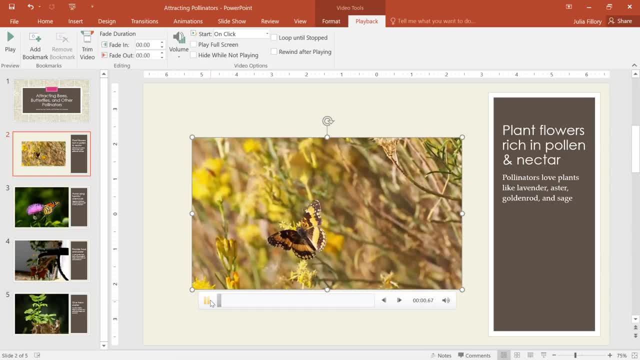 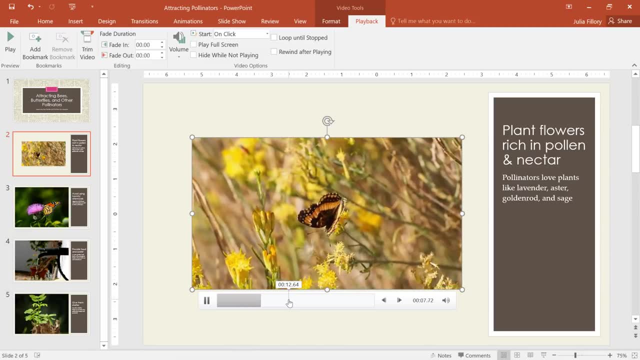 To preview the video, click the Play button here and the timeline to the right will start advancing. If you want to jump to a different spot in the video, click anywhere in the timeline. Let's go ahead and pause for a second so we can take a look at some of the videos we've 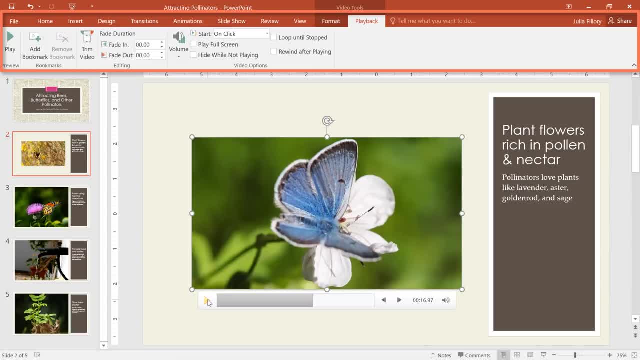 created. Let's look at the options on the Playback tab. Here you can control things that have to do with the way your video is played. You can even do some simple editing. Say you only want to use part of the video, for example, not the entire thing. You can easily create. 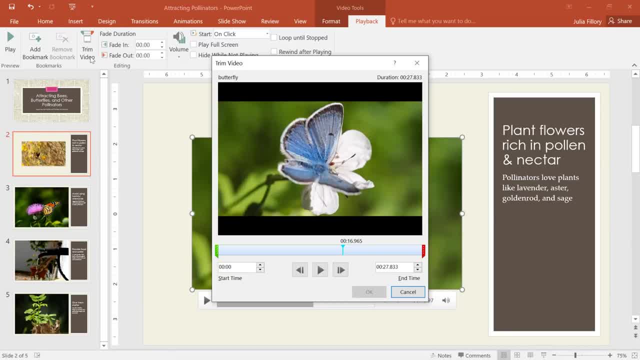 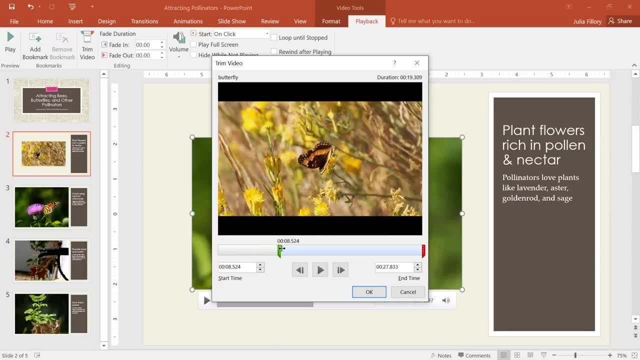 an excerpt using the Trim Video command. Just look for the little green and red markers inside the dialog box. You can click and drag these to change the start and end times. I'm only going to use a few seconds from the end in this case. 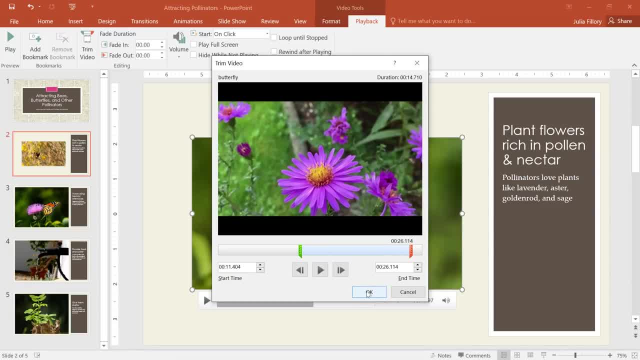 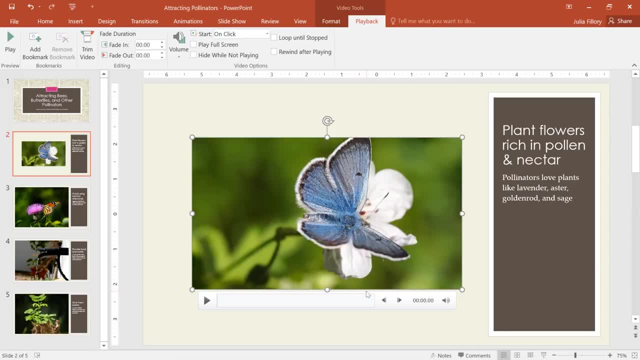 When you're done, click OK and the video will be trimmed to the excerpt you chose. You can also add bookmarks to the video which you can use to jump to specific points during your presentation. All you have to do is click the timeline to mark the point you want to.